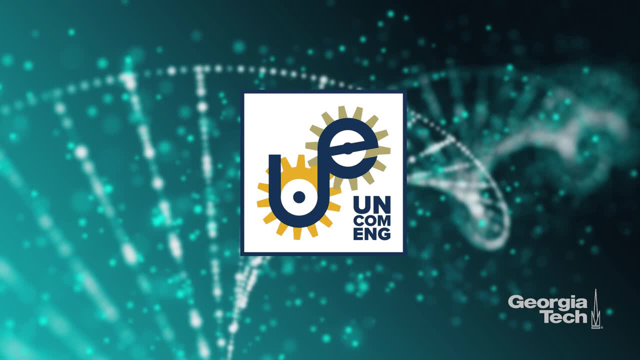 this field. right now, The potential for gene therapies is tremendous Because they treat disease by going after the root source, which is the genetics itself. I think that gene therapies can be subdivided into three buckets. In one bucket, the goal is to produce a lot of the gene. In this case, the disease would be caused by not making enough. 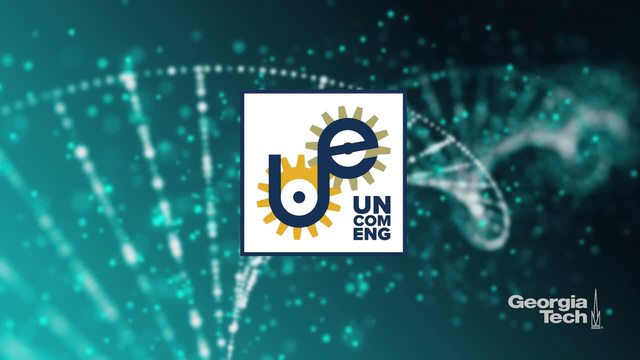 The second bucket is designed to turn off genes- In this case, the disease would be caused by producing too much- And in the third bucket you're actually going in and editing the genome itself. This is the newest form of genetic disease And it's a very new form of genetic disease. 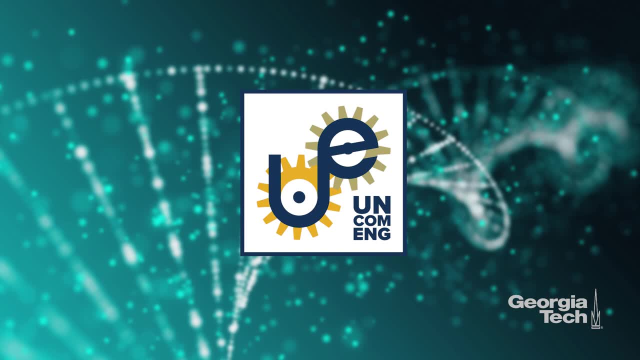 And it's a very new form of genetic disease. And it's a very new form of genetic disease, But it still has some promise. There are many other examples. Some of the work that we perform in my laboratory is designed again to solve a very simple problem. If you want a genetic 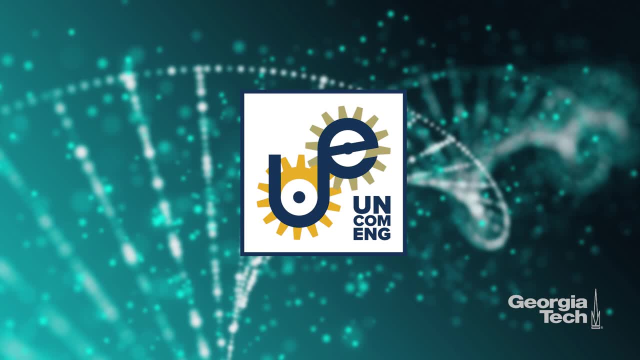 therapy to work, you need to get it to the right cell type. If you have cystic fibrosis and you want to change gene expression in the lung in order to treat the disease, you want that drug to go to the lung. You don't want it to go everywhere else. Once again, the simple problem. 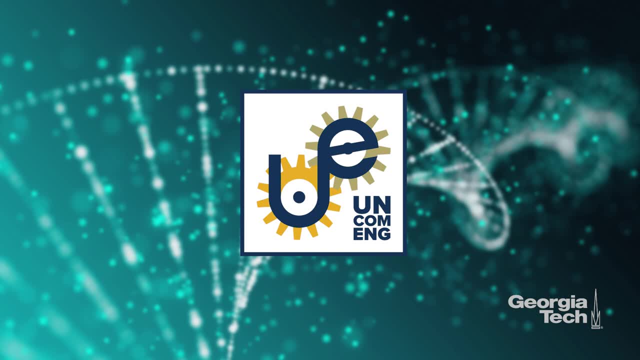 of getting the drug to the right place. at its best is to get it to the right place, And that's an engineering problem. One of the things you talked about was turning off or silencing a gene. Before you talk about the specific therapies, can you give us a little bit of primer on what that really means? 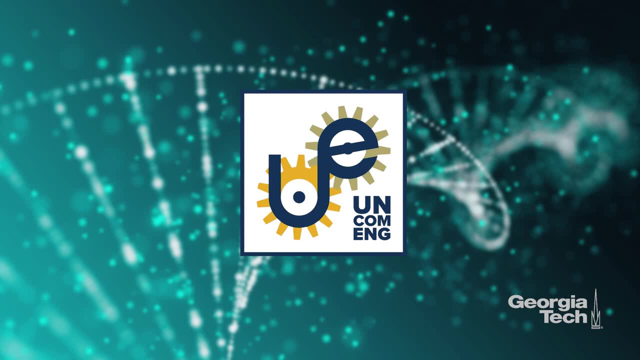 The easiest way to explain this is to go back to sort of biology 101. And that is: DNA makes RNA, which makes protein. So the DNA is like the blueprint. It's what makes you you, And the DNA's job, or one of its jobs, is to make you you, And the DNA's job, or one of its jobs, is to make you. 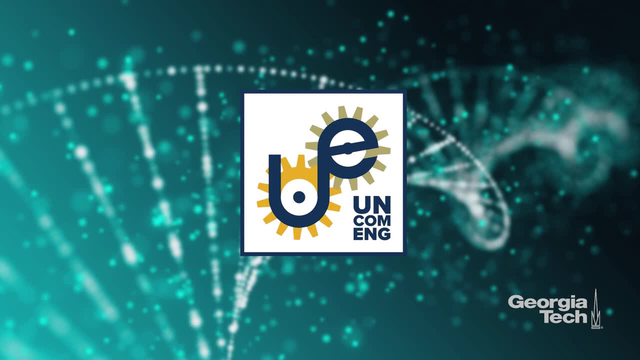 you And the DNA's job or one of its jobs is to make you you And the DNA's job, or one of its jobs is to produce protein, which really does the work. So a DNA will encode for a certain protein If the DNA 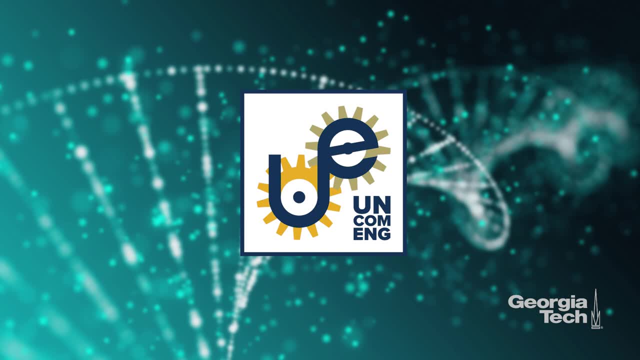 gets a mutation in it, it will encode for the wrong protein and that protein can cause disease. In the case of shutting off a gene, what we're really doing is shutting off the protein production, And we can do this at two different levels. The first level is shutting off the RNA production. 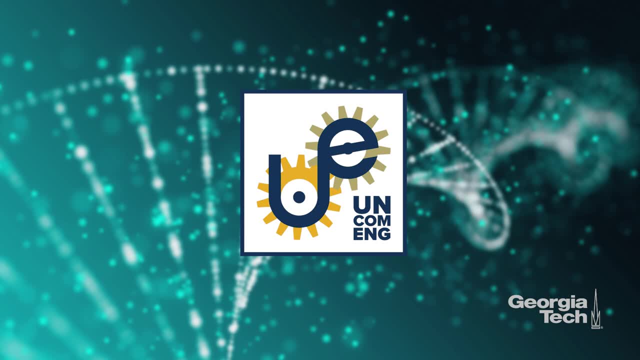 And the second level is by changing the DNA itself. The most advanced clinical trials so far work at the RNA level. They aren't quite there yet with the DNA stuff. Can you say a little bit about your own work and the kinds of things that are going on in your lab? 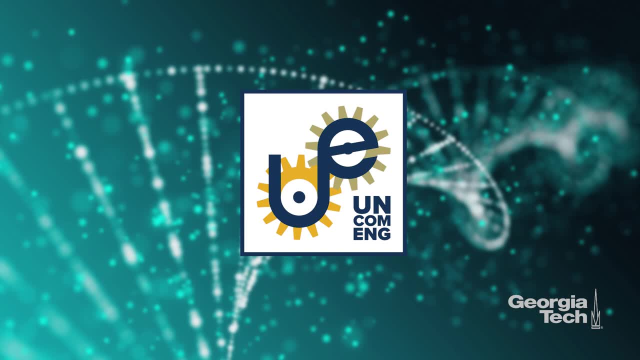 regarding silencing or turning off genes and what's the application. It's a really exciting time to be a scientist in gene therapy right now. My lab focuses on one simple problem: How do we get the drug to go to the right place? 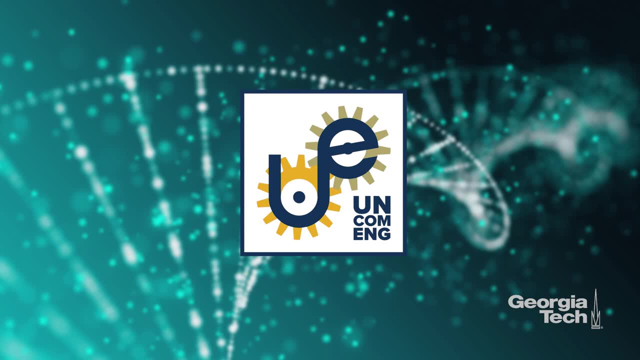 This problem lies at the interface of chemistry, of what we call nanotechnology, and biology, because we are packaging drugs Inside nanoparticles, which are just very small particles, in order to get them to go to the right tissue and to protect them from being degraded and attacked by your body. So my lab focuses on 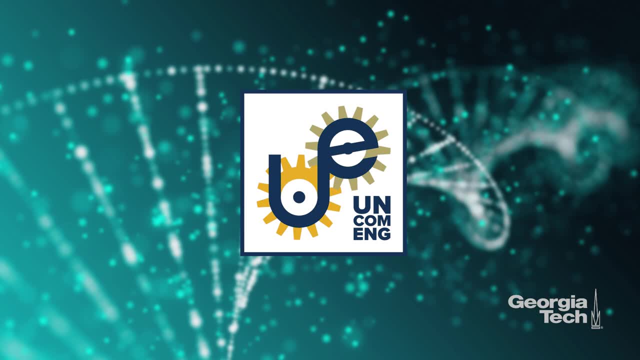 developing nanoparticles that target genetic drugs to the right tissue. A nanoparticle is simply a small particle. I'm about six feet tall and I am 1.8 billion nanometers tall. The systems that we create are about 50 nanometers in diameter. They're little spheres. We package the genetic 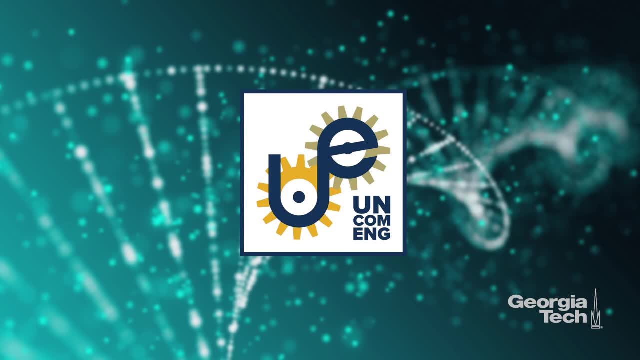 drugs, whether it's DNA or RNA, inside these little spheres and the nanoparticles act as almost mail carriers that take them to the right cell type- the diseased cell type- and help them avoid healthy tissues. This reduces side effects and it improves drug efficacy. 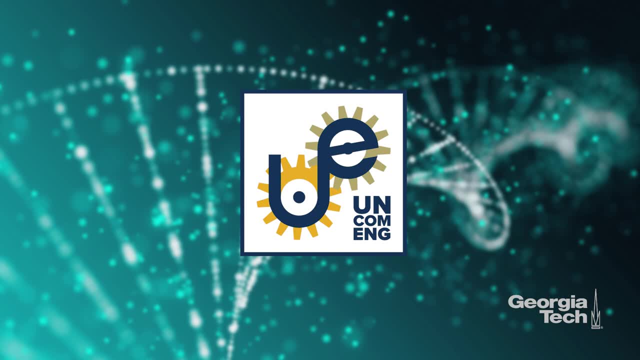 So I'm kind of imagining these nanoparticles in a with the, you know, with the therapies or drugs inside of them, and somehow they get into your body and they're going throughout the body. How do they know where the right place to go is? And 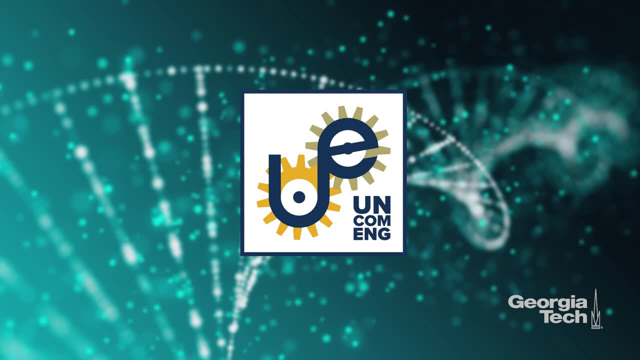 then, once they find the right place to go, how do they then deliver the therapies to the tissue or the cells? It's another great question, and again it lies right at the interface of chemistry and biology and engineering. When you take an aspirin, the aspirin doesn't have flippers. 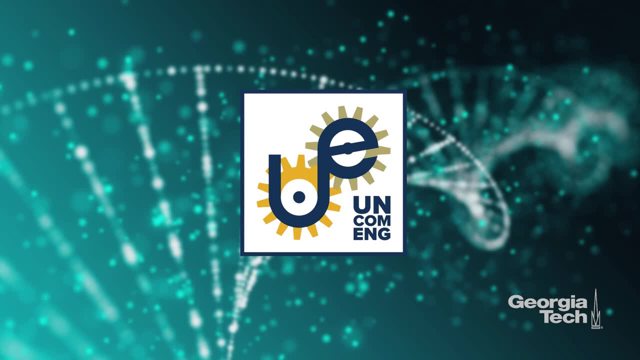 or heat-seeking technology that goes right to your headache. It kind of goes everywhere When you take a genetic drug. if you didn't target it in any way, it would do the same thing. So the way I would think about this is: you can divide the process into two steps. The first step, 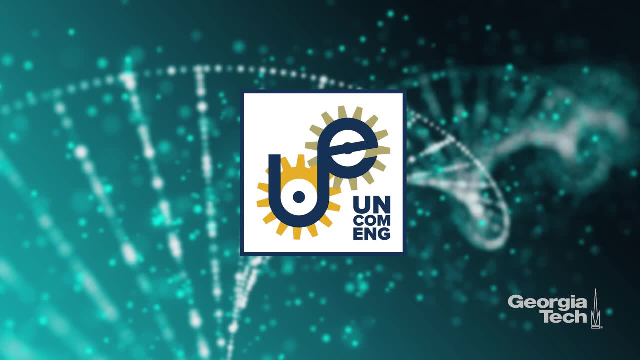 is getting to the right tissue. So just imagine that you're a nanoparticle. You get, you know you're minding your own business, but suddenly you get injected into this bloodstream. The bloodstream is chock full of proteins and lipids and all sorts of stuff- Your bloodstream. 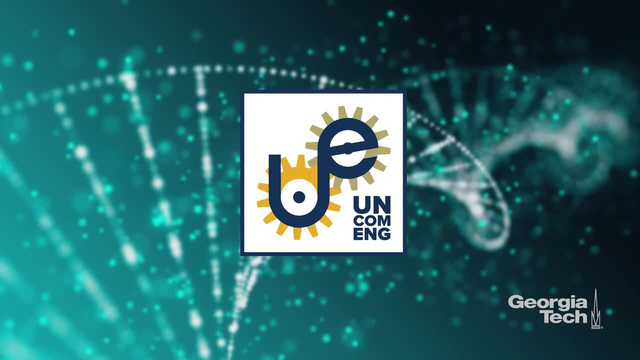 blood isn't just water. It's like a soup that's full of all these biomolecules. So you may interact with some of the biomolecules, but you're passing by the heart, you're passing by the lung, you're passing by the pancreas, the liver, all these organs and every organ is going to look a little. 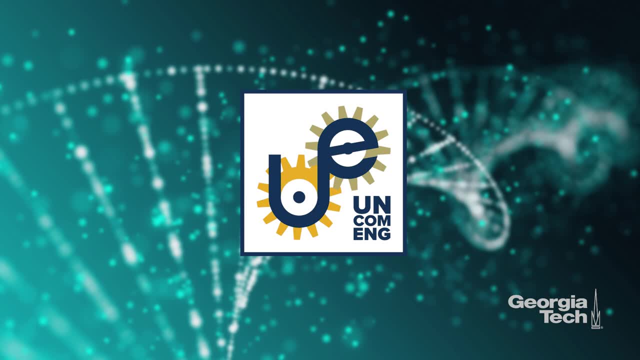 different to you. If we design the nanoparticle the right way, let's say for cystic fibrosis, where you want to target the lung, we design it in a way that the lung looks better to you than the liver, or the lung looks better to you than the kidney, And so you end up in the lung. 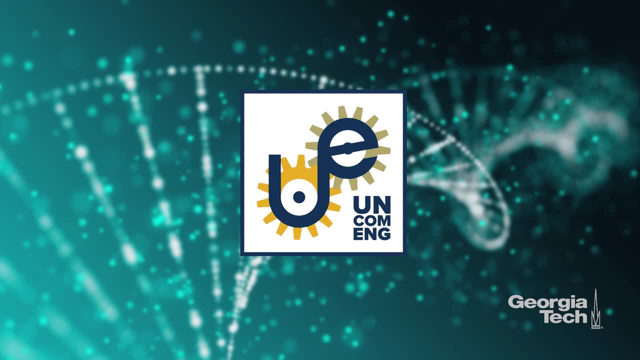 more. so That's the first step: getting to the right place. Once you get there, there's a second, very exciting and interesting step, which is getting into the cell itself. So, although the biology and the biological processes that govern this are still somewhat unclear, we do know a few. 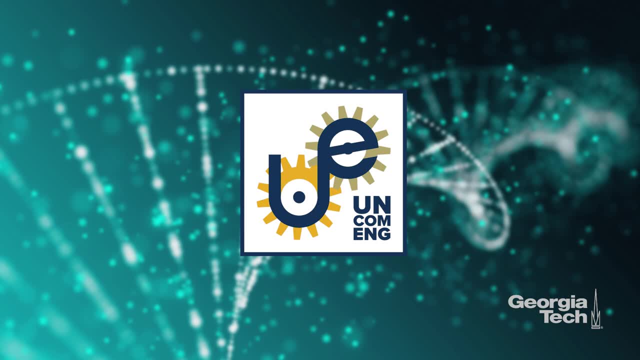 things, which is that cells gobble things up actively, Just like us. cells need nutrients and they get nutrients from their environment, from their neighborhood, if you will, and from the bloodstream. So cells gobble stuff up very actively. Ideally, your nanoparticle is designed. 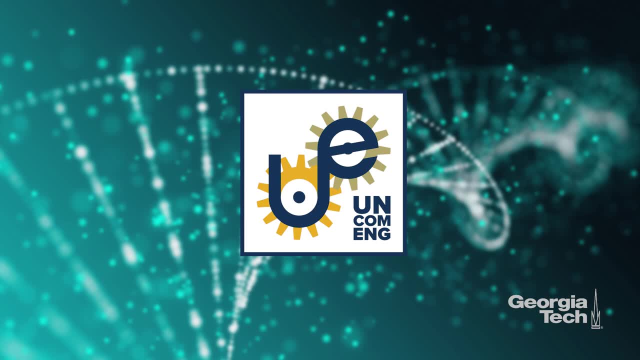 in such a way, with such a chemistry that makes it tasty to cells, so they end up gobbling it up. This allows the drug to get into the cellwork and do its job. So again I would sort of divide it into two parts: First getting to the right tissue and then second getting into the cell. 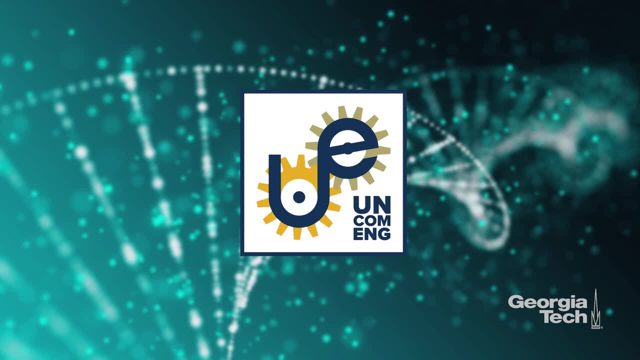 once it's at the tissue. So the delivery of the nanoparticles to the cells, that really is a big part of the process. So how do you get the nanoparticles to the cells Sounds like an engineering problem. Can you say more about the drug delivery? 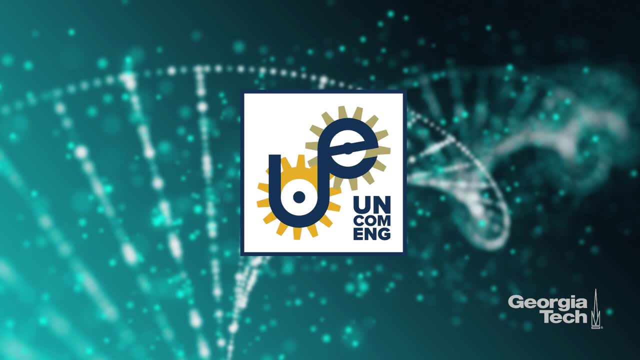 because it's so specifically targeted What your students are doing with that. My students are developing what we call DNA barcoding technologies, And the easy way to think about this is: we've developed technologies that allow us to perform a few thousand experiments all at once. The technology behind it is pretty fun. Think about it this way: We can make a giant. 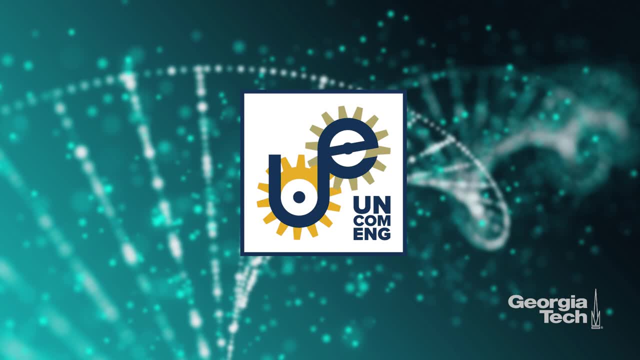 library of nanoparticles. Nanoparticle one, nanoparticle two. nanoparticle three. nanoparticle two might be small. Nanoparticle two might be large. Nanoparticle three might have a positive charge on it. Nanoparticle four might have a negative charge on it. We can make thousands. 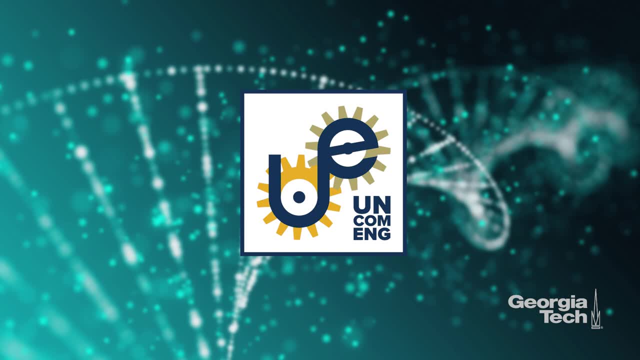 of different nanoparticles, of different chemical structures. We don't know which ones are going to work. So how can we test thousands? Well, the way we do it is we use DNA as a molecular tag. So nanoparticle one gets DNA barcode one. All that means is nanoparticle one carries. 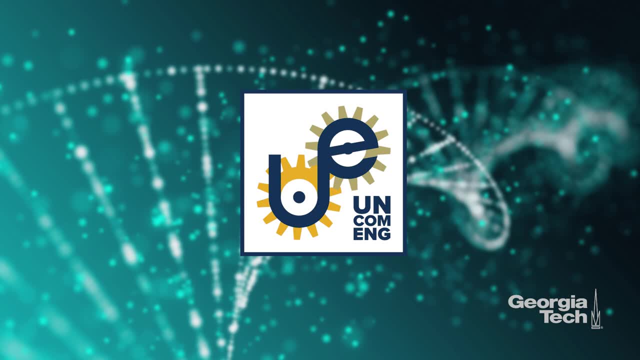 instead of carrying a drug to turn off a gene, it just carries the drug to the cell. So we carries a little tag. That's a DNA sequence that we know. Nanoparticle two carries a different DNA tag- just a different sequence, again that we know. And you can do this many times in a day. 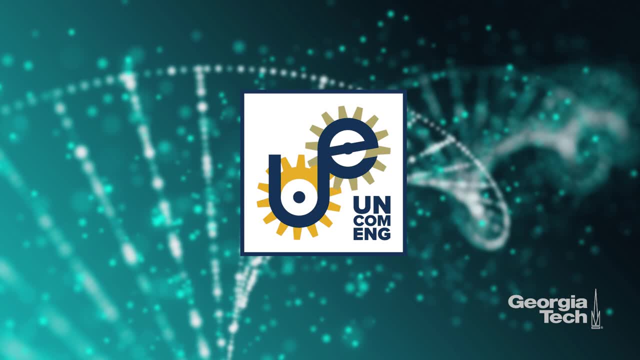 My students have made up to 250 nanoparticles, each with its own molecular tag, in a day. You can then mix all the particles together and administer them in a single experiment. You then isolate the DNA and you can use deep sequencing- Again this technique that you know: you spit in a tube and 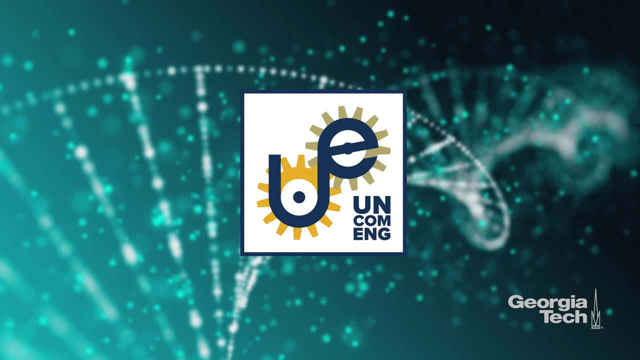 send it to Ancestrycom or to 23andMe. We use that same machine, the DNA sequencing machine, to analyze how all those DNA sequences behaved at once. So if you do 250 different nanoparticles of 250 sequences and you run your experiment and you take out the cells and it turns out that 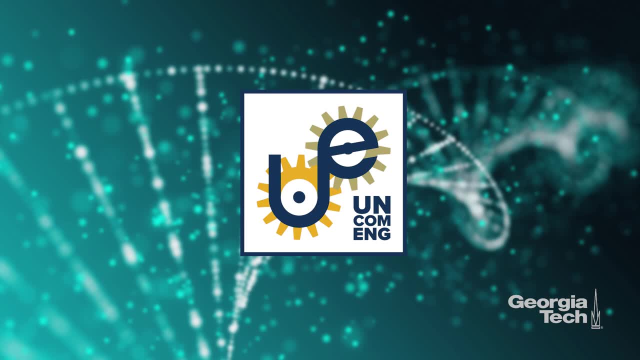 barcode number 17 shows up in those cells more so than the other barcodes. that means that nanoparticle number 17 shows up in those cells. So if you do 250 different nanoparticles of 250 might do a good job. So this allows us to perform hundreds and thousands of experiments. 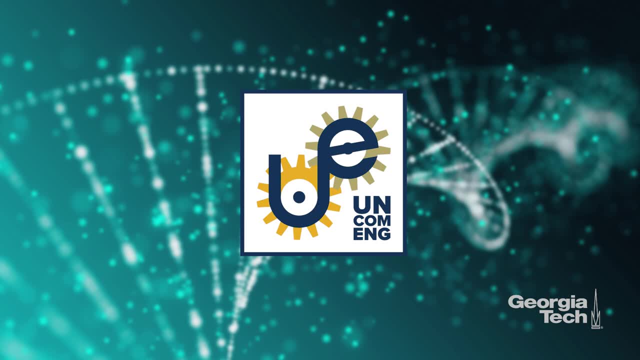 simultaneously And actually using this process, we've been able to identify nanoparticles that do target new tissues and new cell types, So it's pretty efficient. I think we can accelerate the development of drugs this way, So let me get this right. This is incredible. So you know, I think 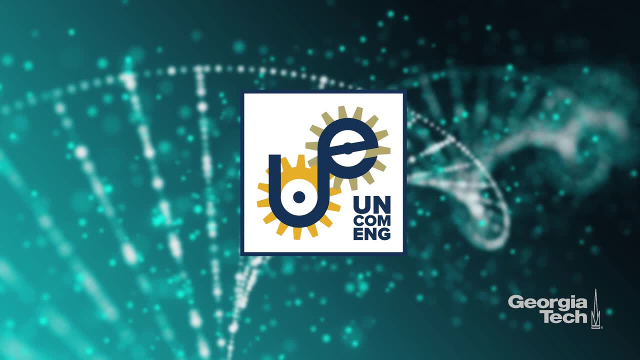 the way that people have done experiments for hundreds of years is they try one thing at a time, they try one therapy at a time and you then test that therapy. You're saying now you can do that same thing. Instead of testing one therapy at a time, you can test hundreds or thousands of. 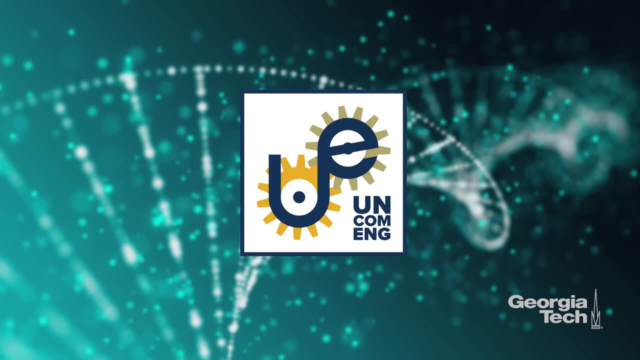 therapies at a time, And I guess your goal is in this case. it's about the delivery of the nanoparticle into the cell, And all then you need to do is to read out and then examine the cell and see which of the nanoparticles got through. Do I have that right? Yes, that is exactly right. 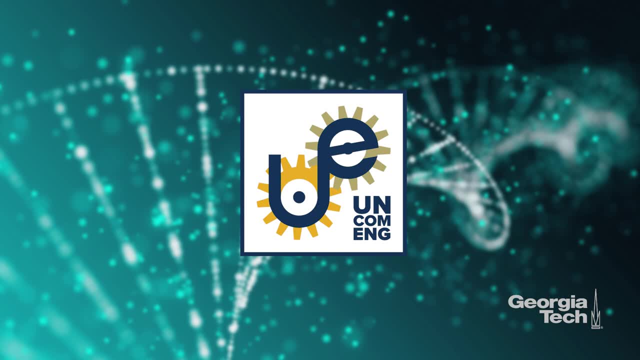 And I can tell you that it is a very exciting time to be in the lab right now, because we I thought of this technology a few years ago. It took a while to engineer it so that it was robust, but it is now working And in a typical 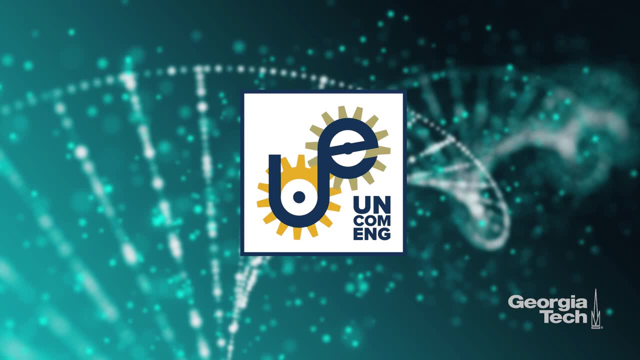 experiment now. one of my students will test about 250 nanoparticles and we'll analyze the delivery to, let's say, 30 cell types. So 250 times 30 is what. Whatever, that is, 7,500 experiments performed at once. 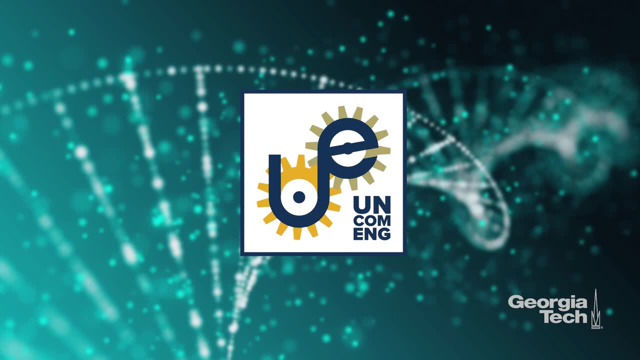 The data sets that we're generating now are so big and so much bigger than anything I've reported in my career- that we actually had to develop a bioinformatics pipeline to analyze the data sets because there was no pipeline in my field to analyze it. It's pretty fun, because what you 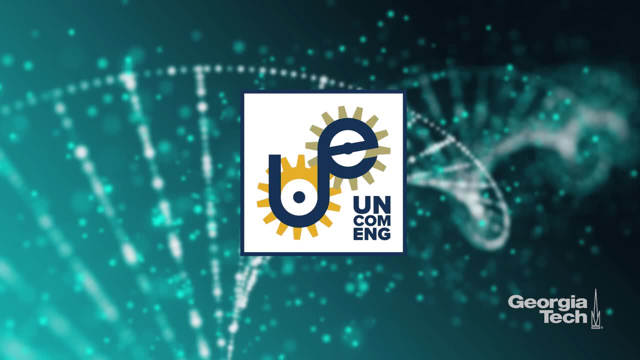 can find is that, let's say, nanoparticle 17 does well in lung cells, but really doesn't do well in heart cells. Well, that's great, because you can have specific delivery to the lung And so we can measure delivery to our target tissues as well as all of our. 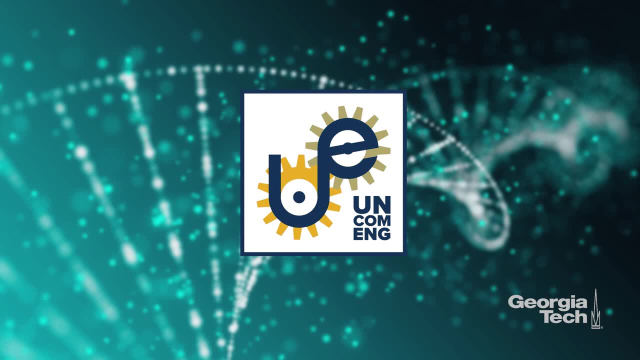 what we call side effect tissues or off-target tissues, in a single experiment. So we can do years of work, basically in three days, And this is, I think, a real step function change in the ability to do these experiments. We are interested in commercializing this in order to get products. 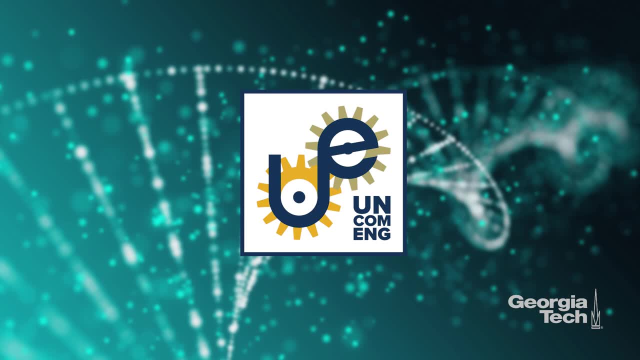 to patients more quickly. The ultimate goal is to accelerate the development of genetic therapies, And I think that this platform really does stand a chance to do that. We know that we've received a lot of interest from the field so far, from companies that are already in the clinic, in fact. 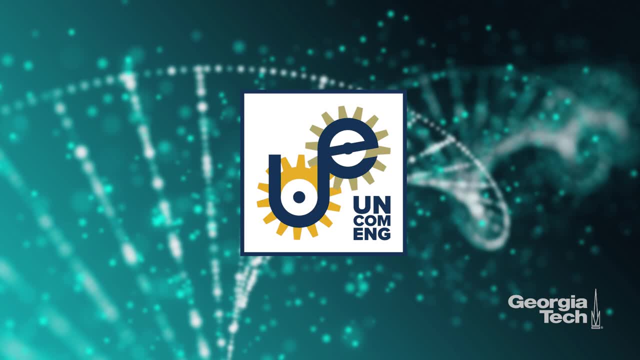 And they view this technology as very promising and a way to accelerate how quickly genetic therapies actually make it into clinical trials and actually make it into patients. So we're really excited about all of these opportunities. So the idea of barcoding, you know, nanoparticles- 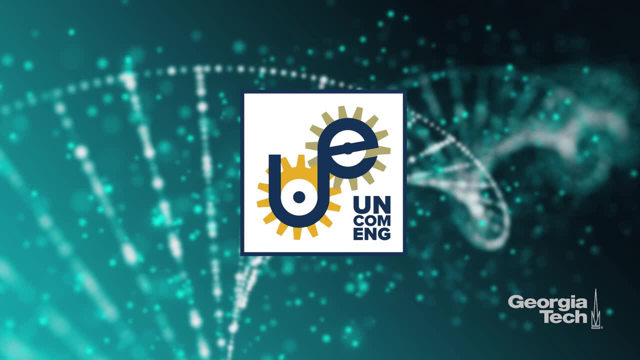 to get to tissues for addressing disease is absolutely fascinating. How close is this to actually being able to do that? How close is this to actually being able to do that? So I do think our work has implications for human disease. I'll give you an example that 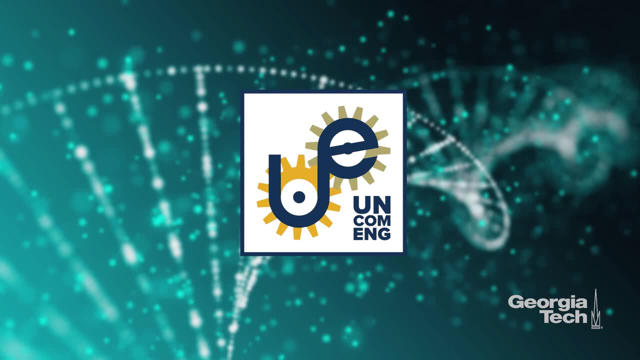 it's pretty exciting. right now We have initiated a collaboration at the National Cancer Institute outside DC And this collaboration is with a surgeon. This surgeon does this very cool thing: He operates on patients that have liver cancer. He would do it anyway. It's part of the normal procedure And after he does the surgery to remove 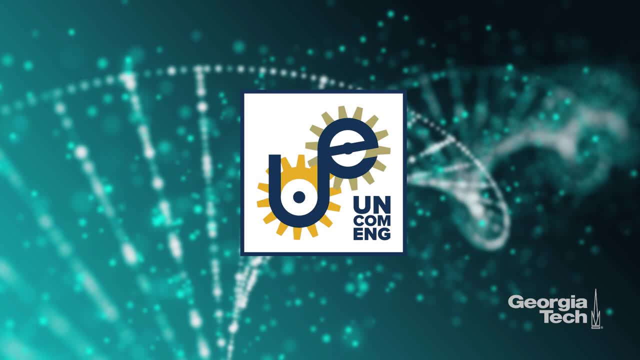 the tumor. he actually made a machine that keeps the tumors alive for about a week And, as you can imagine, these things are very rare samples and they need to be treated with respect. So one of the advantages to our system is we can essentially perform a few hundred experiments using one. 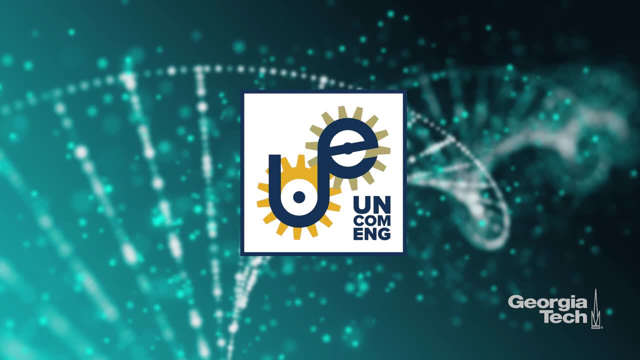 patient tumor, instead of performing one experiment with one patient tumor, And although we haven't started these experiments with him yet, I am hopeful that we'll be able to start experiments like this where we're screening directly in patient samples, maybe within the next two years. 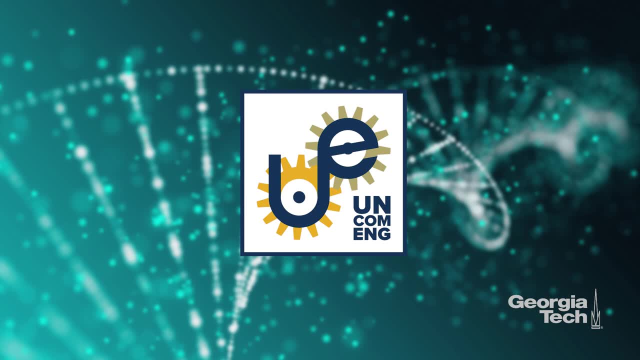 That would be great. I think the key point here is that when you're dealing with patient samples, and so I think it actually is an advantage of our system that we can test hundreds of things per sample instead of one thing per sample. So you talked about the three different. 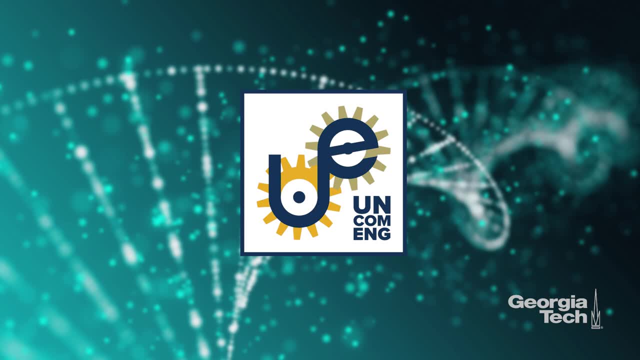 approaches to GDL, One of which was gene editing. I've heard about this technology called CRISPR, About what CRISPR is and the kind of work that's going on in your lab. CRISPR is arguably the most exciting biotechnology discovery, certainly of the 21st century so far. 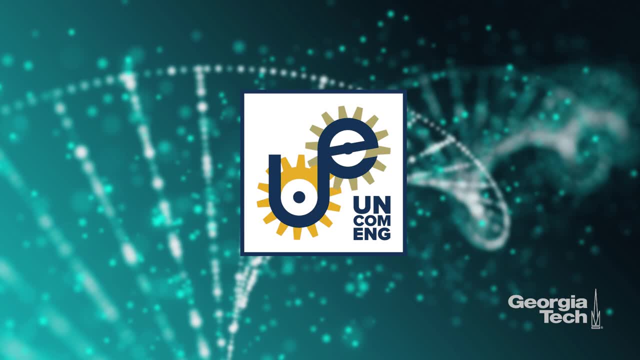 Put succinctly, CRISPR allows us to edit the genome very easily. Even five years ago, if you wanted to take DNA and change the DNA sequence, you could do it using things called zinc fingers, Zinc fingers and talons, but it was going to take a lot of money. It was going to take a lot of time. 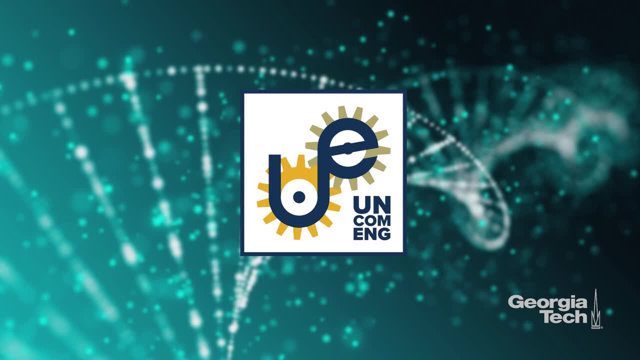 CRISPR does the same thing as zinc fingers and talons: It edits DNA, it changes DNA sequences, but it's really really easy to use. And so now, for the very first time, scientists can do something as simple as edit 10 different genes, 100 different genes, and see which gene causes. 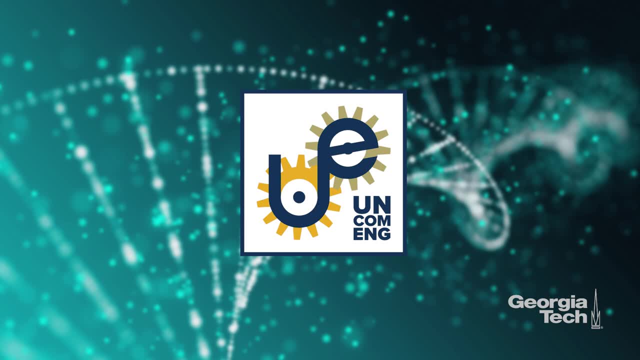 a tumor to grow. You can accelerate these scientific studies. Therapeutically, CRISPR can be used to edit cells so that they target tumors more effectively, And in the future, CRISPR may be used to edit the genome inside human patients as well, in order to turn off a gene that's causing disease. 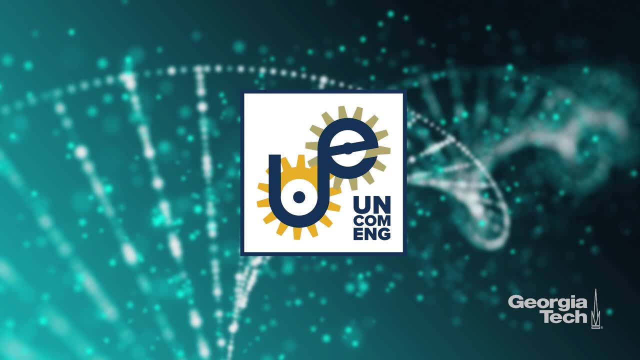 So, from our lab's perspective, we do a lot of work on CRISPR. CRISPR is not going to work unless you get into the right cell, And so, from our perspective, we're just trying to get it into that right cell. 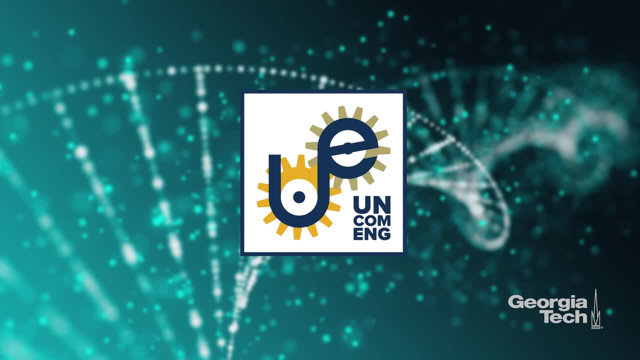 I will say, from a scientific perspective, CRISPR is one of the most, if not the most exciting technological development I've ever been exposed to. It is changing how things are done. I'd like to change directions just a little bit, And here you talk about your own path. 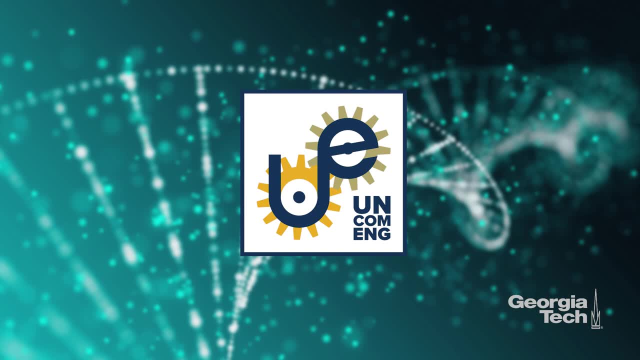 maybe even from junior high or before, how you made your way to Georgia Tech and how you made your way to wanting to study this area and become a biomedical engineer. When I went to MIT and Harvard Medical School for my graduate work, I was in what's called the HST. 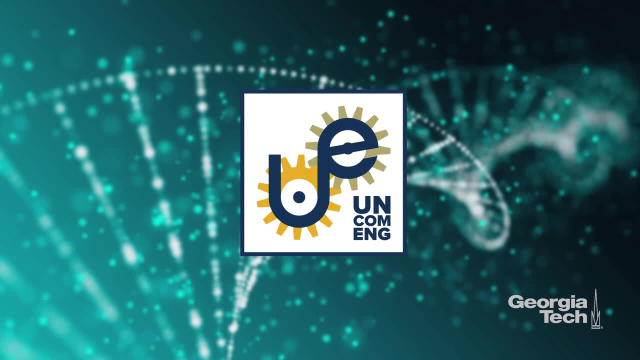 program, I started drifting more towards biology and medicine. So at MIT I did my PhD work in material science. But you're also forced to take two years of medical school at Harvard with the medical school students, And so I remember one very interesting day as a first-year graduate student. 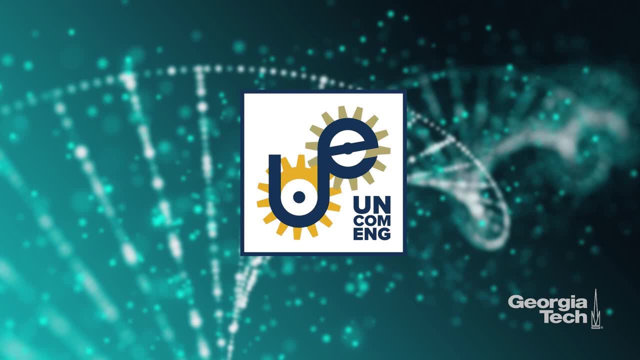 walking out of a pathology exam at the medical school and then walking right into a quantum mechanics exam After taking the bus, it really does stretch your brain a little bit. As I got into the medical school classes, it became clear that biology was just so elegant.